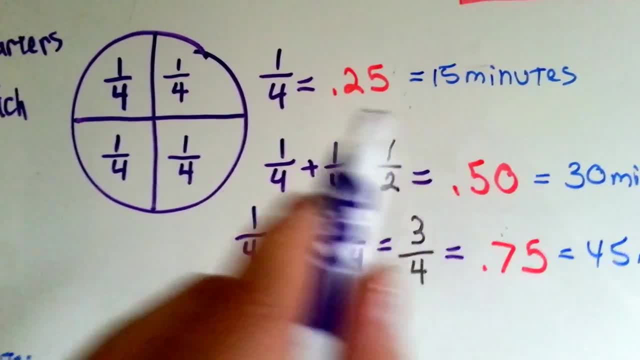 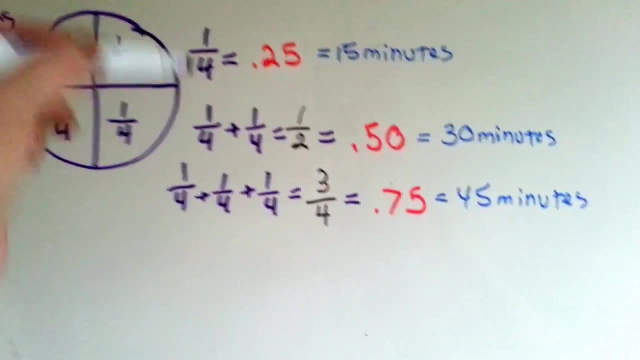 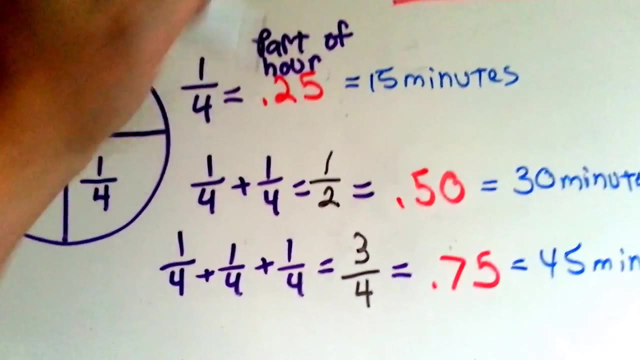 which is equal to 15 minutes. That's where the confusion comes in. okay, That's not the minutes. That's the part of the hour. okay, It's one-quarter of an hour. It's 0.25 of an hour If you put two of these together. 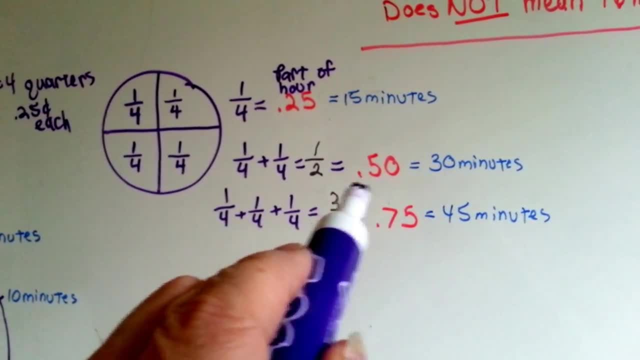 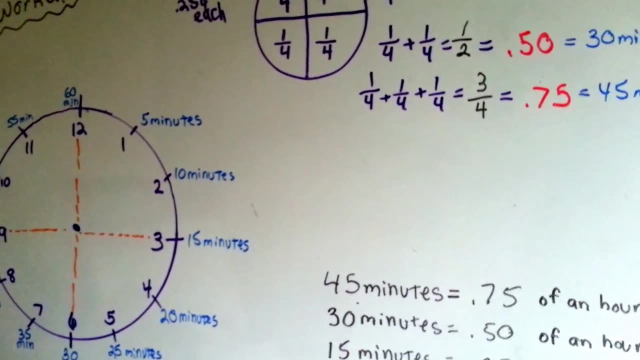 it would make half an hour, which would be 0.5, which would be 30 minutes. right, When it's down in the six it's at 30 minutes. okay, If you were to count three of these: one-fourth plus one-fourth plus one-fourth. 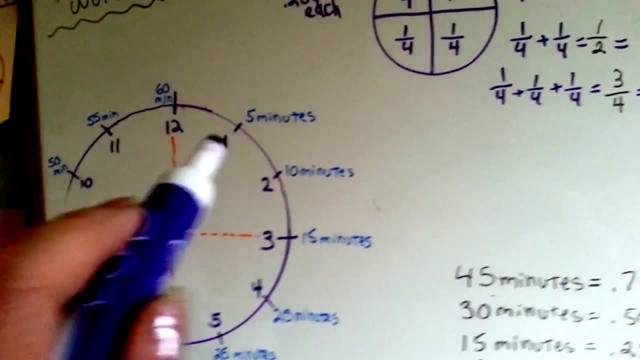 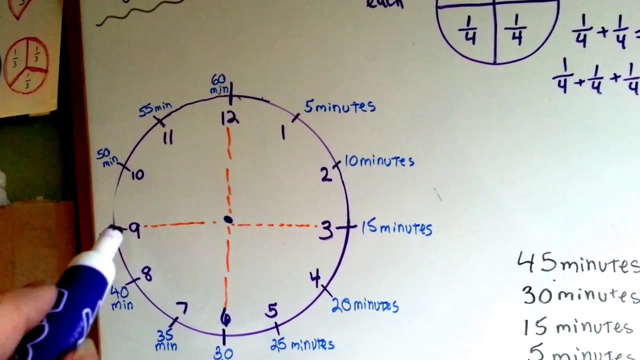 it would equal three-quarters, three-fourths, And three-fourths is 45 minutes. If you know how to tell time, you know that when the minute hand is pointing to the nine that it's on the 45. You would say it's 2.45 in the afternoon or 6.45 in the evening. 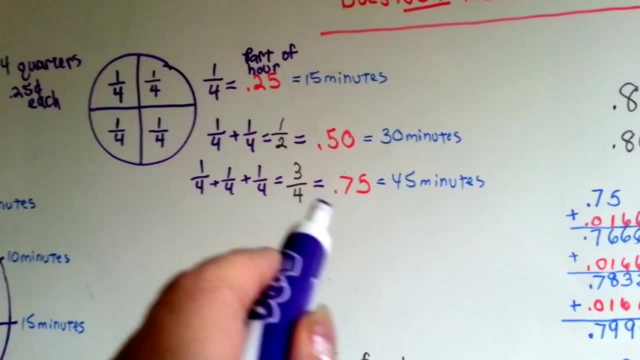 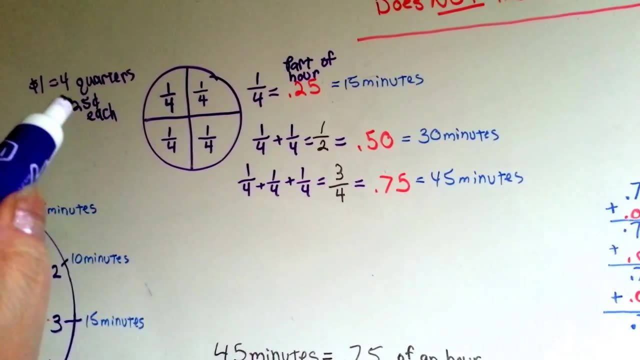 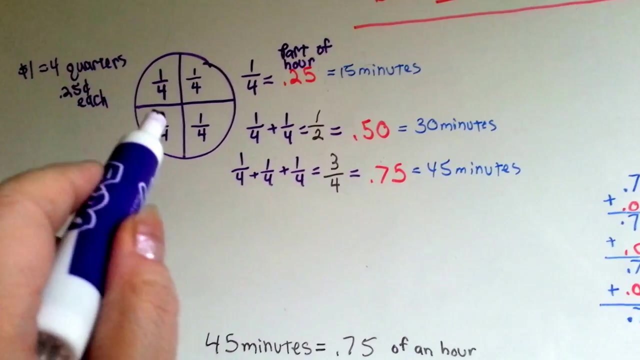 So that three-fourths is equal to 0.75.. It would be like having three-quarters three pieces of 25 cents. You would have 75 cents, But that three-fourths- that 0.75, is equal to 45 minutes. okay. 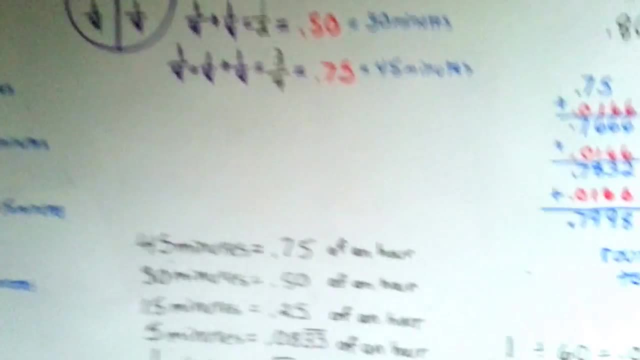 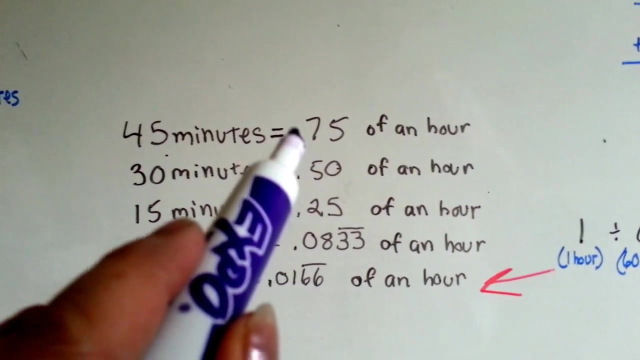 So how can someone work 16.8 hours? Well, let's look at this. We now know that 45 minutes is three-quarters of an hour, 0.75 of an hour. 30 minutes is 0.5.. That's a half an hour. 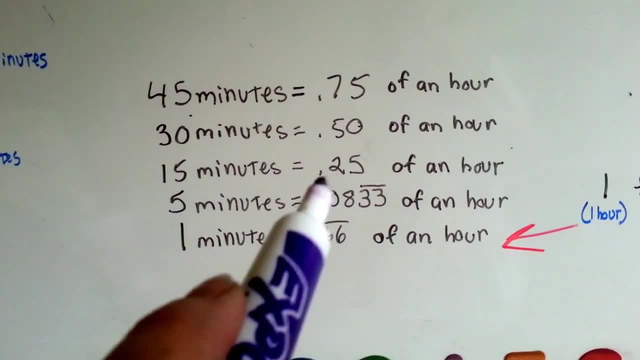 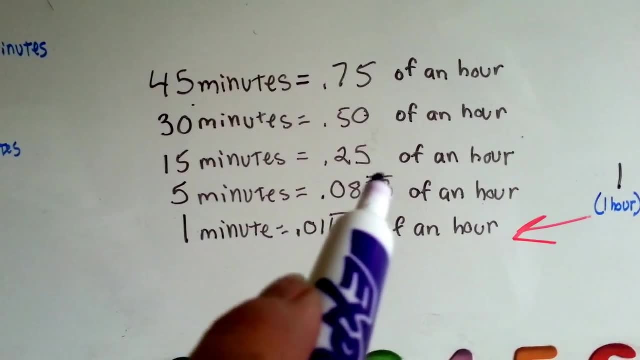 15 minutes is a fourth of an hour, like a quarter: 0.25.. Five minutes would be 0.0833.. Now the reason the line is above here is because the three goes on for a long time and that's a way of saying the three repeats okay. 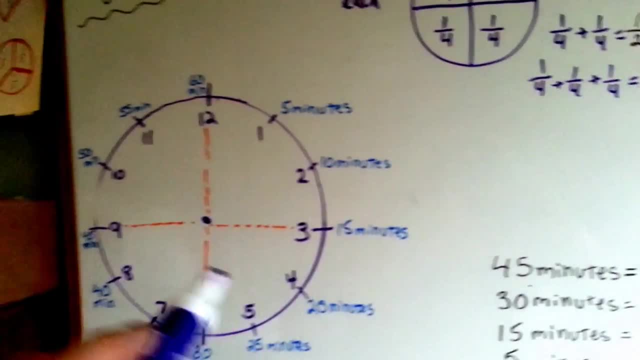 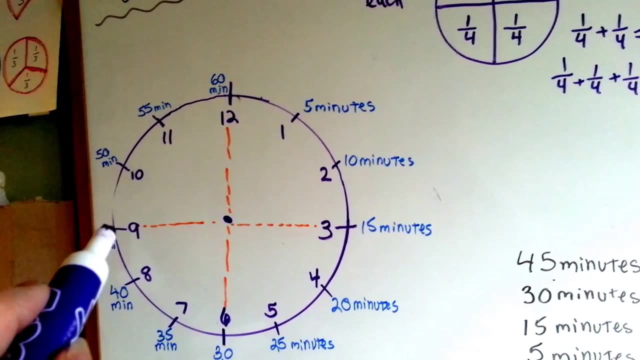 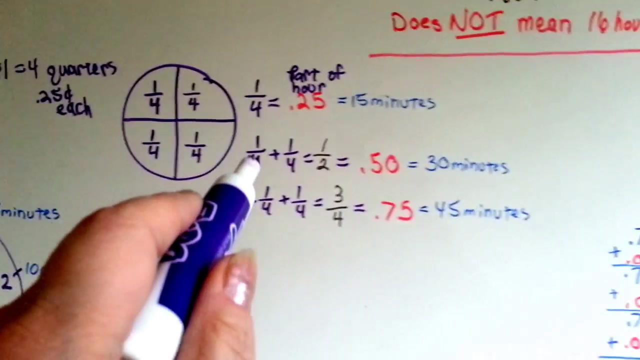 equal three-quarters, three-fourths And three-fourths is 45 minutes. If you know how to tell time, you know that when the minute hand is pointing to the nine that it's on the 45. You would say it's 2.45 in the afternoon or 6.45 in the evening, So that three-fourths is equal. 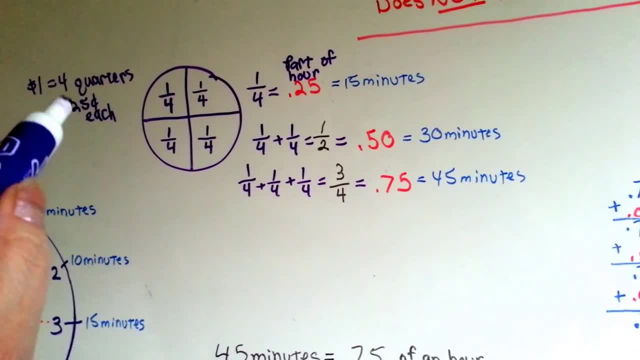 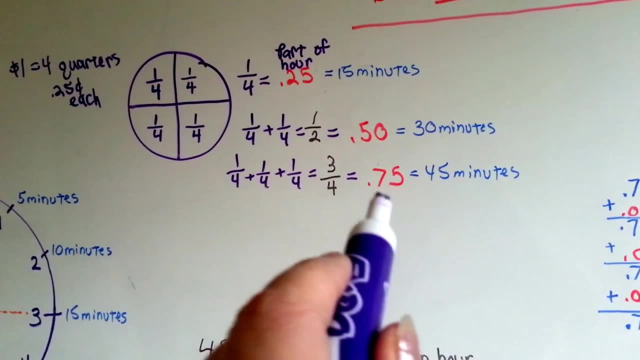 to 0.75.. It would be like having you know three-quarters, three pieces of 25 cents. You would have 75 cents, But that three-fourths, that 0.75, is equal to 45 minutes, okay. 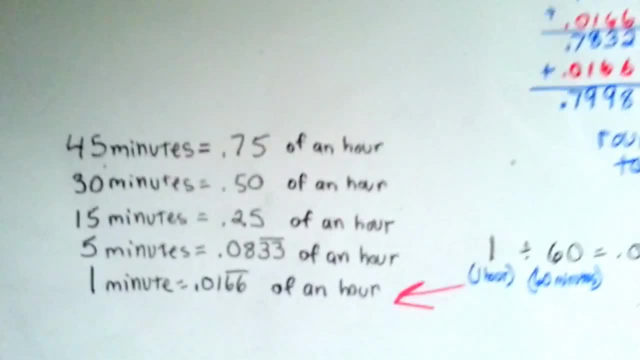 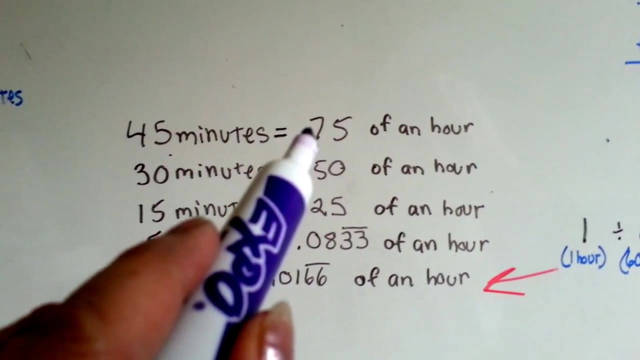 So how can someone work 16.8 hours? Well, let's look at this. We now know that 45 minutes is three-quarters of an hour, 0.75 of an hour. 30 minutes is 0.5, that's a half an hour. 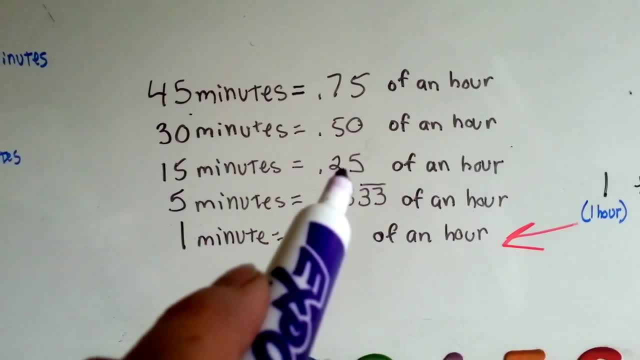 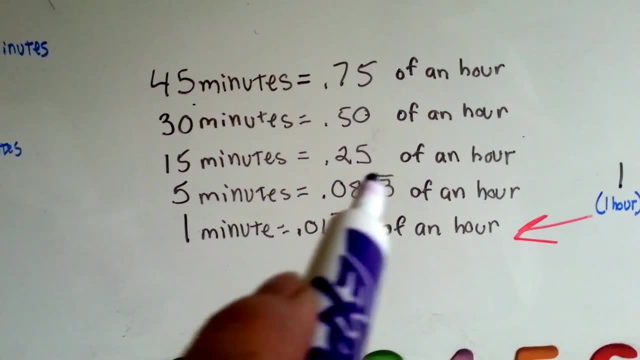 15 minutes is a fourth of an hour, like a quarter: 0.25.. 5 minutes would be 0.0833.. Now, the reason the line is above here is because the three goes on for a long time and that's a way. 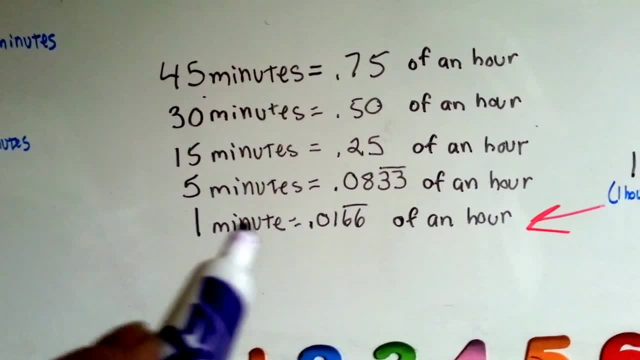 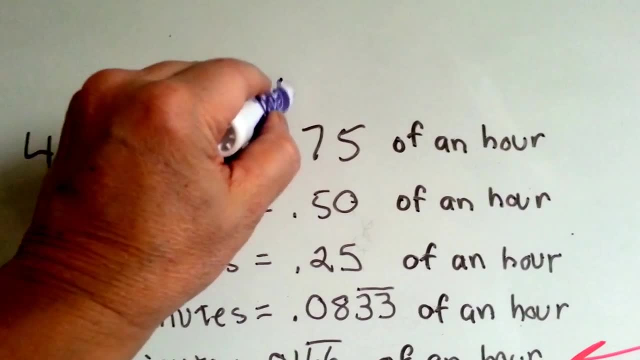 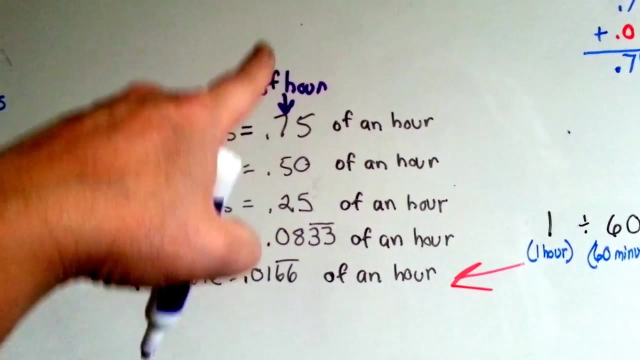 of saying the three repeats: okay, One minute turns out to be 0.0166 of an hour. okay, This is how much of the hour. okay, It's not money, it's how much of the hour. a decimal point of the hour worked, So one. 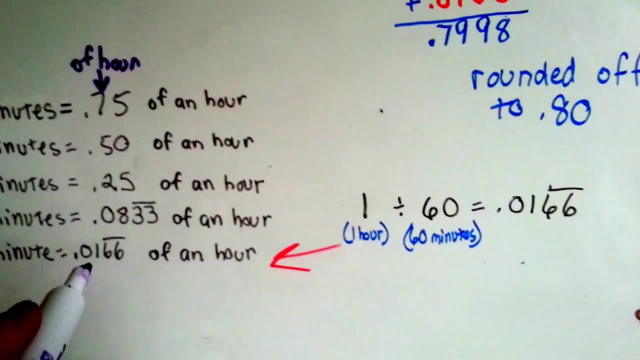 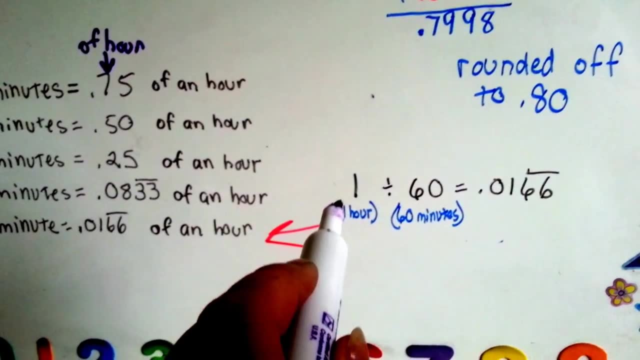 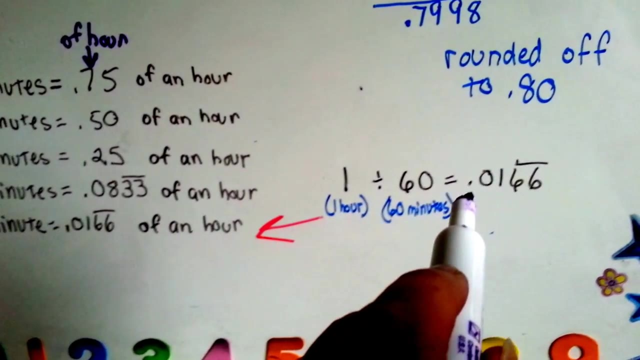 minute is 0.0166.. The way to find that out is: you take, you go in your calculator and you put one for one hour divided by 60,, 60 minutes, and it comes out to 0.0166, and. 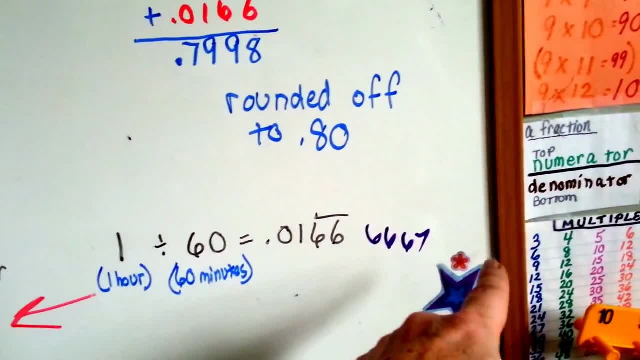 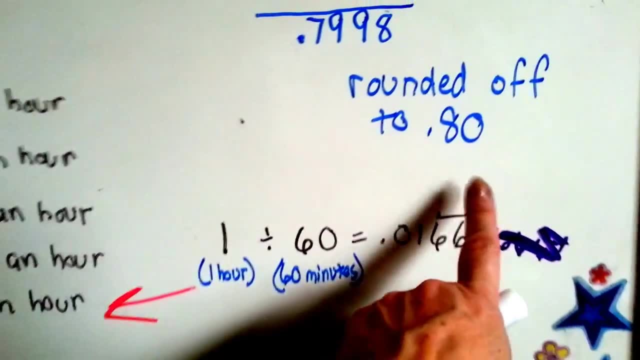 actually it says 6667.. Or something like that. it goes on, but I didn't count those and I just stopped it there and put the line there. okay, So you can actually just do this 0.016.. So let's. 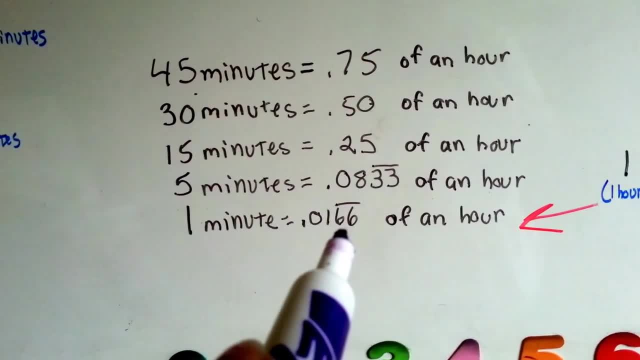 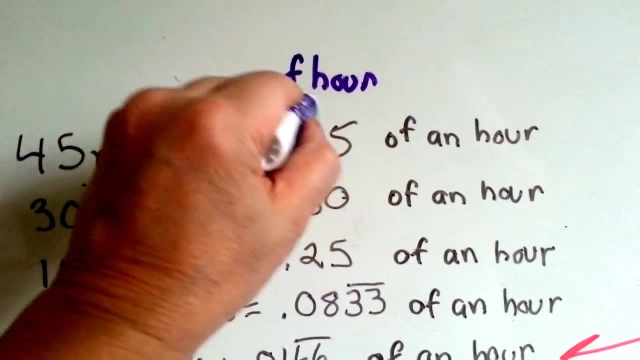 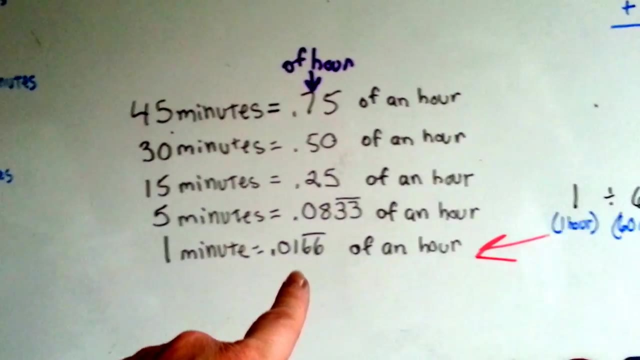 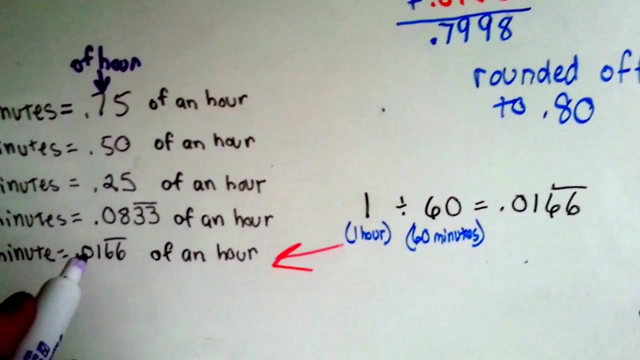 One minute turns out to be 0.0166 of an hour. okay, This is how much of the hour. okay, It's not money, It's how much of the hour, a decimal point of the hour worked. So one minute is 0.0166. 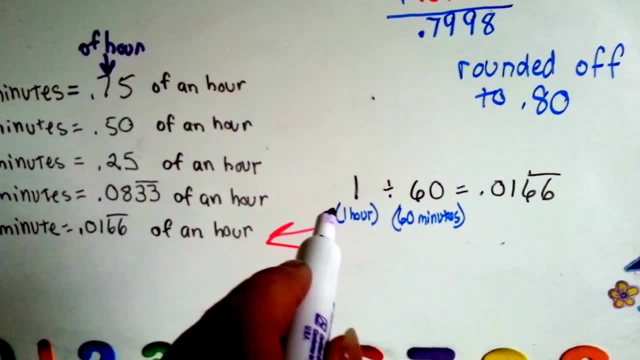 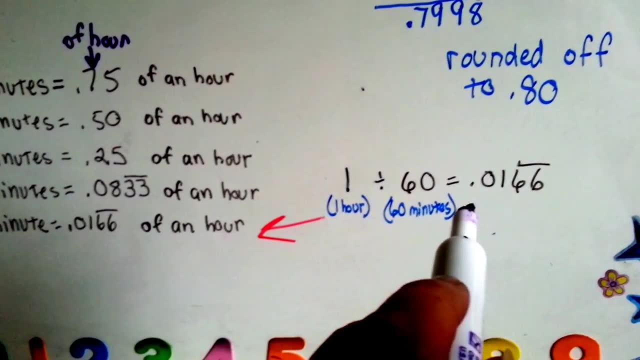 The way to find that out is you take, you go in your calculator and you put one for one hour divided by 60, 60 minutes, And it comes out to 0.0166.. And actually it says 0.0166.. 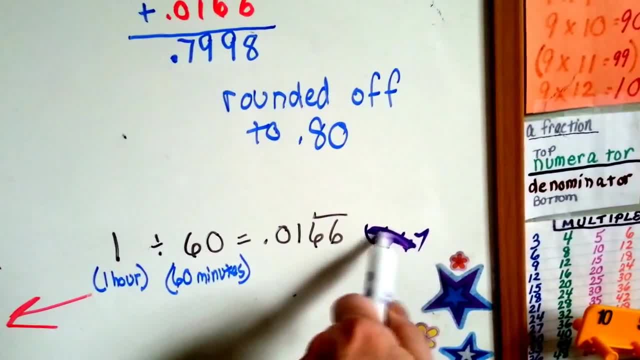 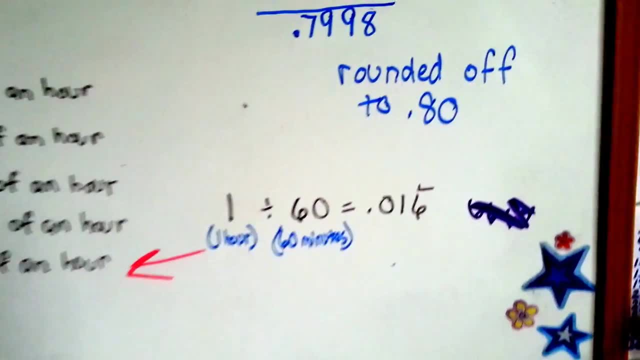 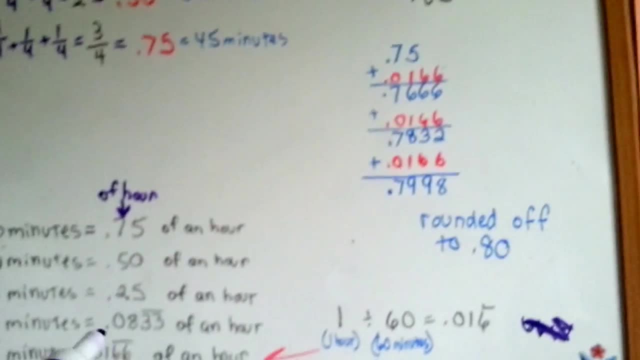 0.067 or something like that. It goes on, but I didn't count those and I just stopped it there and put the line there. okay, So you can actually just do this 0.016.. So let's say we're going to figure out what 0.80 is, all right. 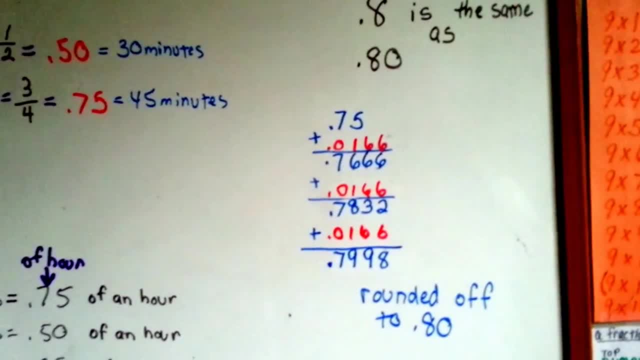 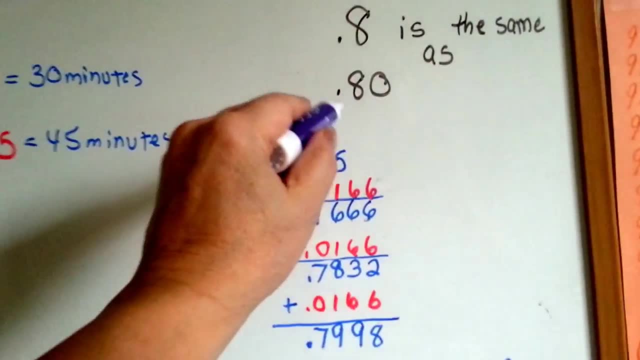 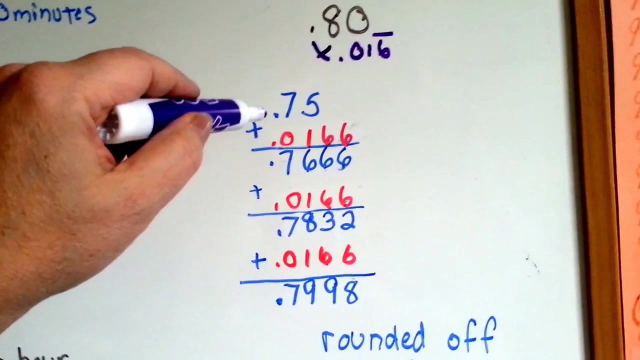 So, pardon my focus there is giving us problems. We're going to find out what 0.80 is Now. you can either do 0.80.. 0.80 times 0.016, or we could do it this easier way. 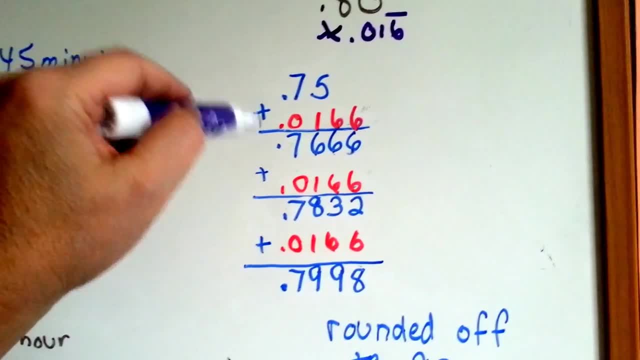 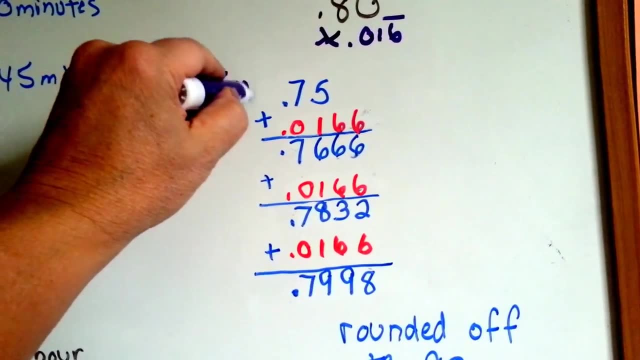 Well, that might be easier really up here, but let's do it this hard way so that you can actually see what's going on. So we're going to take 0.75,. okay, That's 45 minutes, all right. 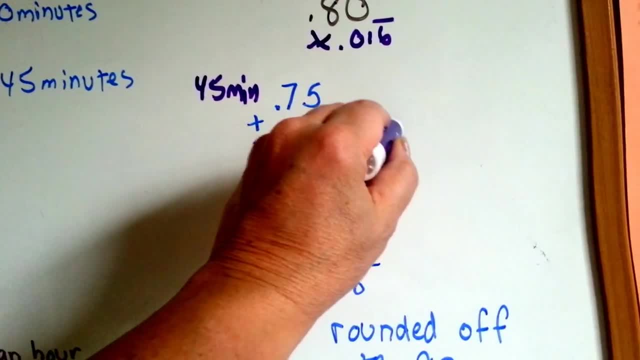 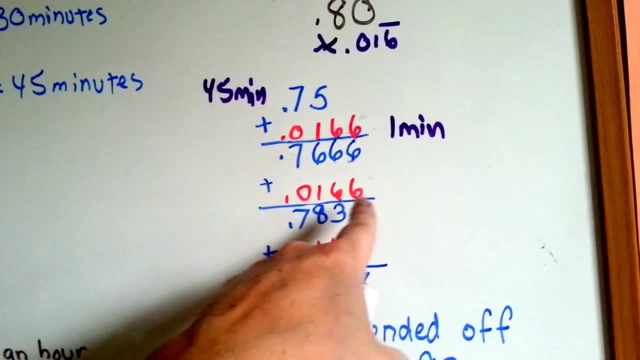 That 0.75.. We're going to add one minute to it. 0.0166, and we're going to get 0.7666.. Let's add another minute. Now we're at 2 minutes, okay. 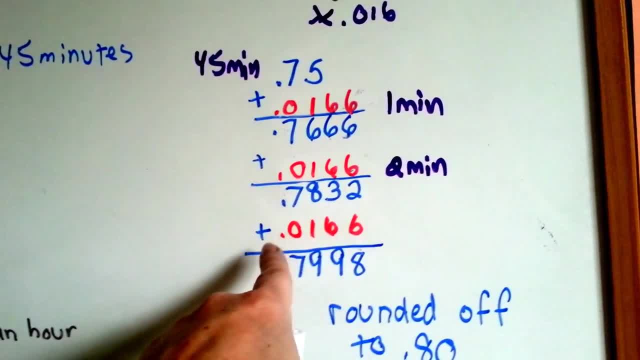 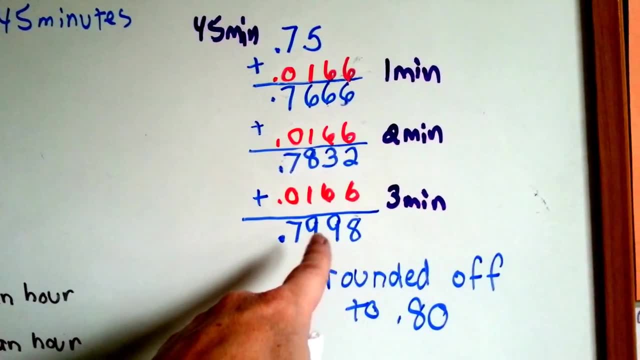 You add it up and it comes to 0.7832.. Let's add another minute. Now we're at 3 minutes that we've added. okay, That comes to 0.7998,. and to round it off, your boss is being nice rounding it off to 8, okay. 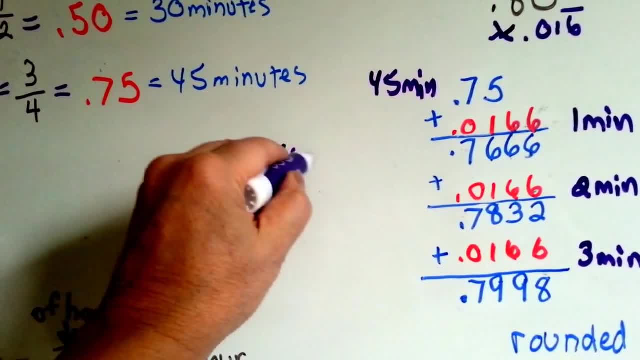 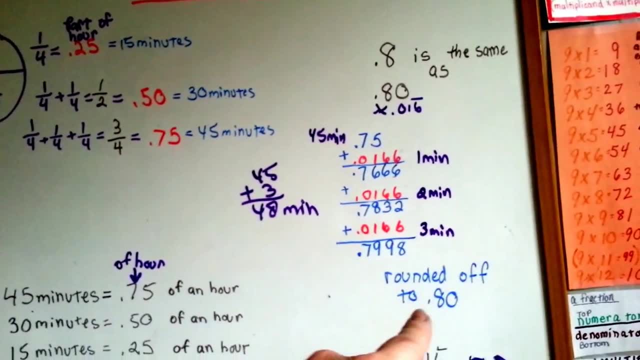 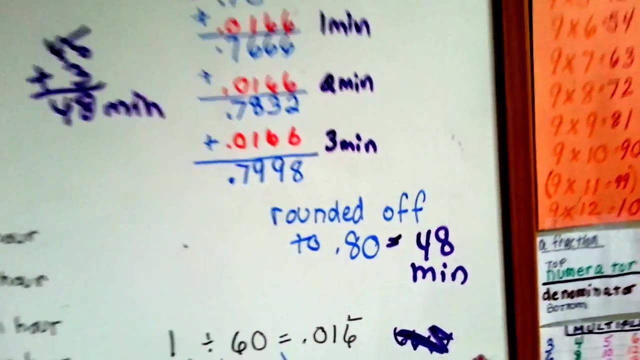 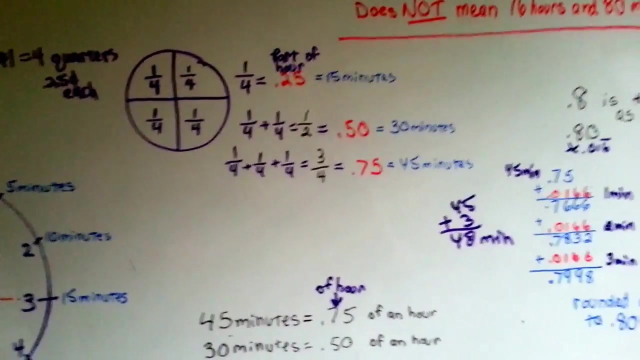 So that's 45 minutes and 3 minutes. That's 48 minutes. So 0.80 is equal to 48 minutes. That means she worked 16 hours and 48 minutes and she would be paid for 16 hours and 48 minutes. 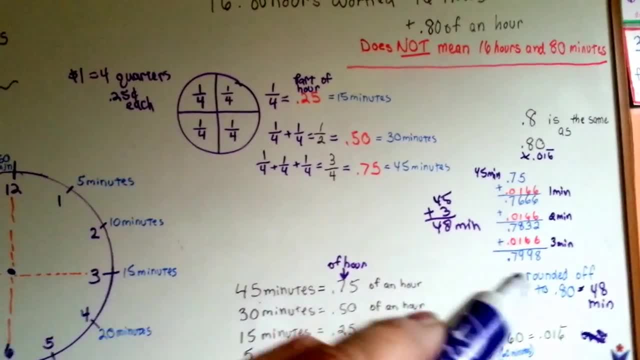 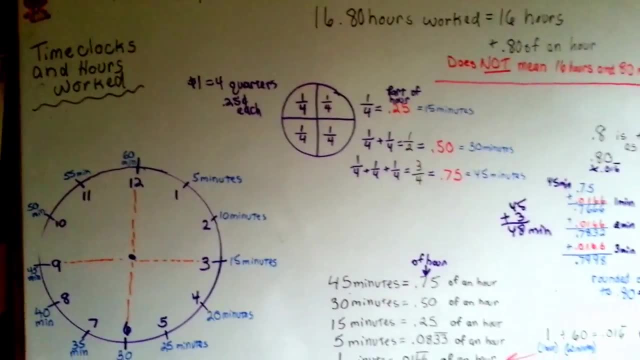 She must have either did a little extra overtime, past the half hour or past the hour, or she got off work 12 minutes early And didn't complete her day by 12 minutes. Either way, to figure out your time and your pay, 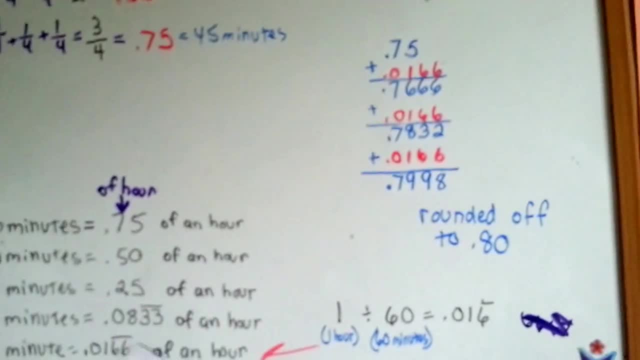 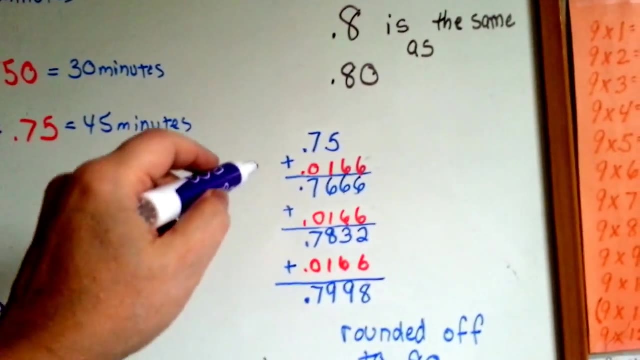 say: we're going to figure out what 0.80 is. alright, So pardon my focus there is giving us problems. We're going to find out what 0.80 is. Now you can either do 0.80, or you. 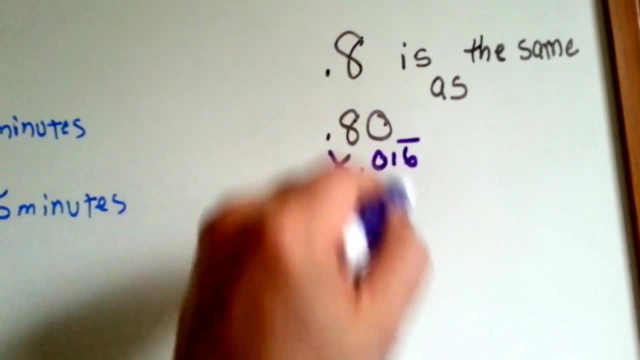 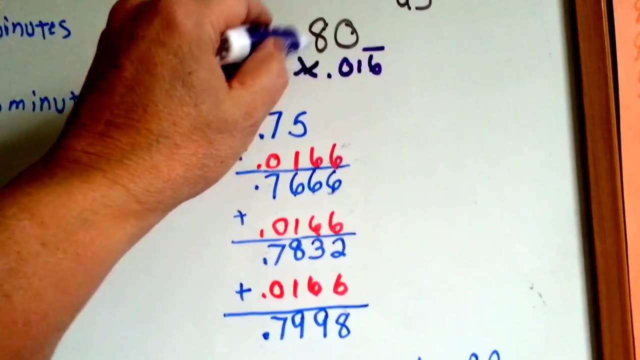 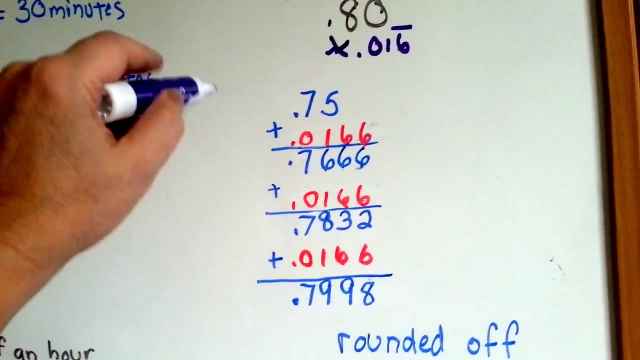 can do 0.80 times 0.016, or we could do it this easier way. Well, that might be easier really up here, but let's do it this hard way so that you can actually see what's going on. So we're going to take 0.75,. okay, That's 45 minutes. alright, That 0.75.. We're going. 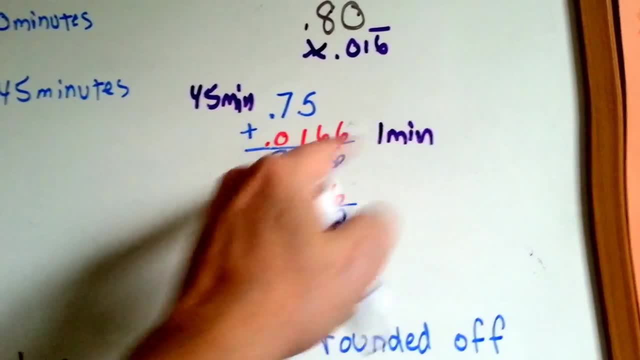 to add one minute to it- 0.0166, and we're going to get 0.775.. So we're going to add 0.0166, and we're going to get 0.775.. So we're going to add 0.0166, and we're going. 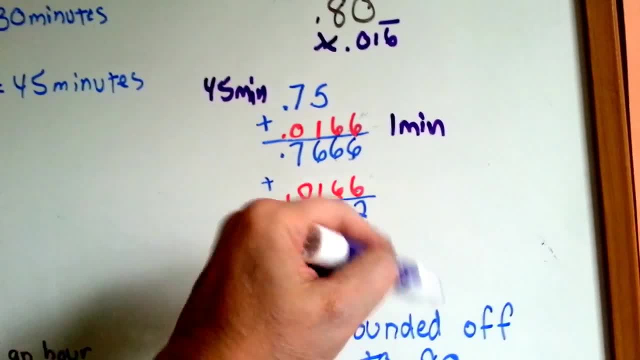 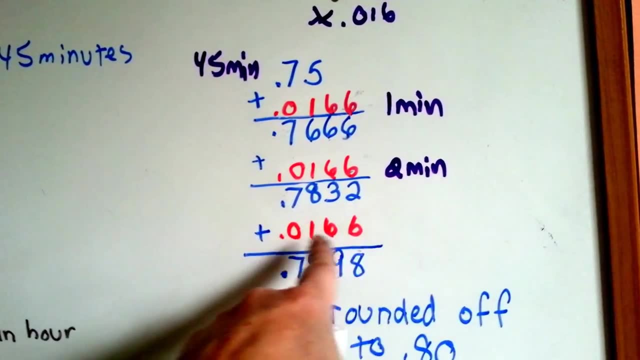 to get 0.7666.. Let's add another minute. Now we're at 2 minutes. okay, You add it up and it comes to 0.7832.. Let's add another minute. Now we're at 3 minutes that we've. 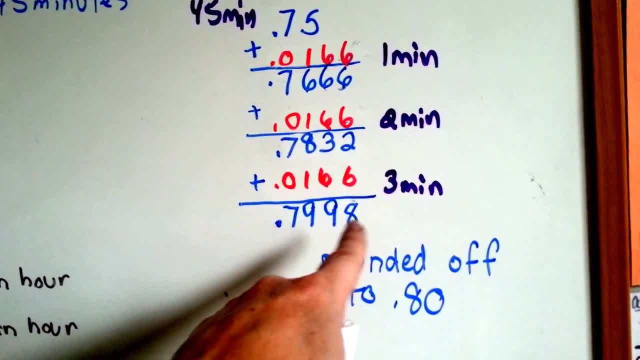 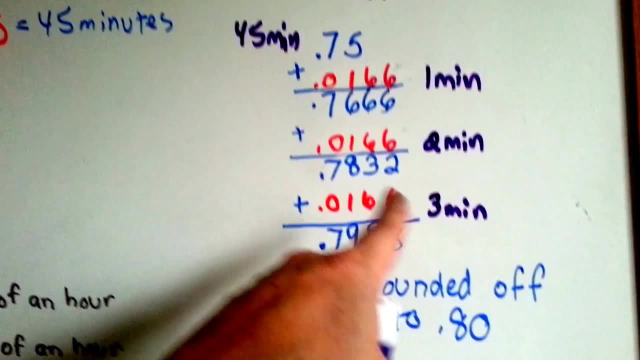 added: okay, That comes to 0.7998,. and to round it off, your boss is being nice rounding it off to 8,. okay, So that's 45 minutes and 3 minutes. So we're going to add another. 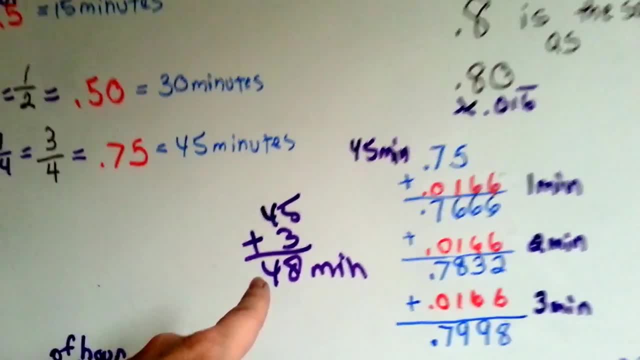 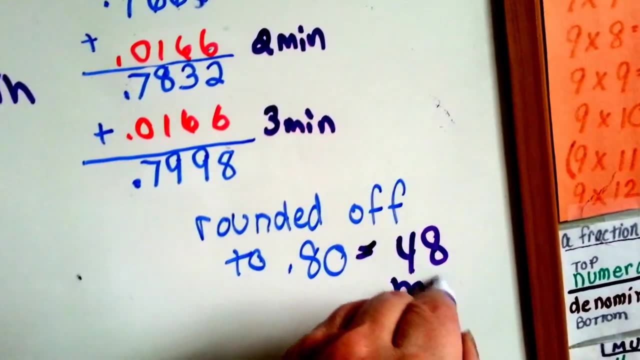 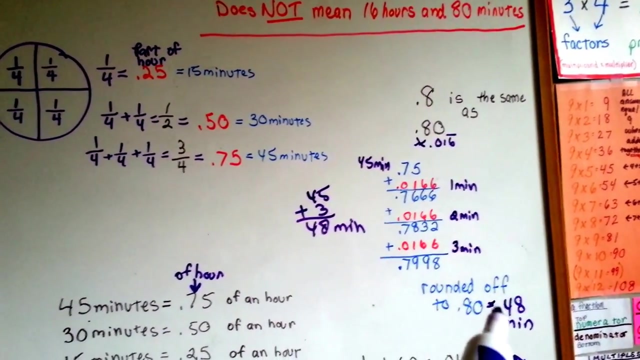 minute. Now we're going to add another minute. Now we're going to add another minute, So let's add a minute. That's 48 minutes. So .80 is equal to 48 minutes. That means she worked 16 hours and 48 minutes and she would be paid for 16 hours and 48 minutes. She must. 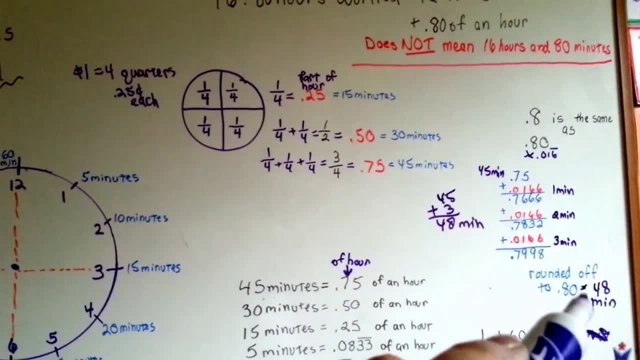 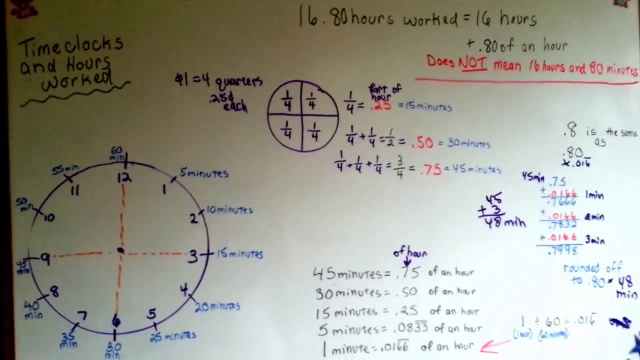 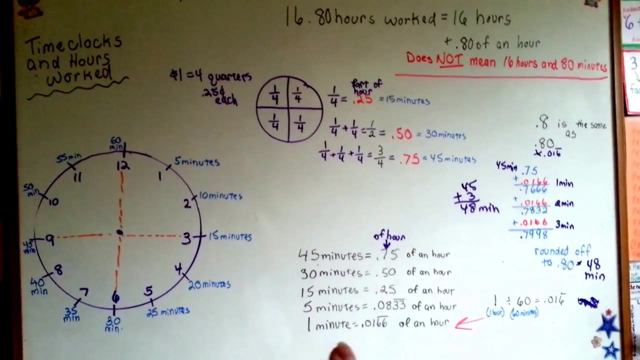 have either did a little extra overtime, passed the half hour or passed the hour, or she got off work 12 minutes early and didn't complete her day by 12 minutes. Either way, to figure out your time and your pay, keep in mind that .0166 is one minute of an hour, and when you see, 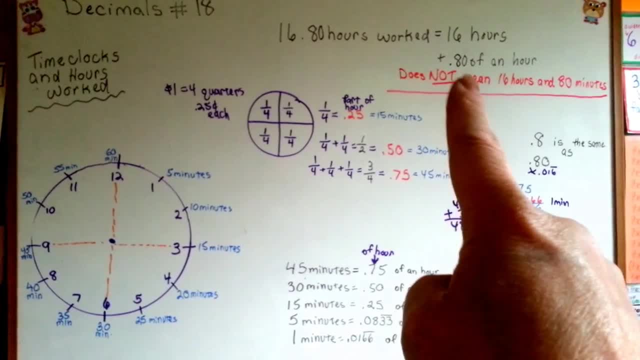 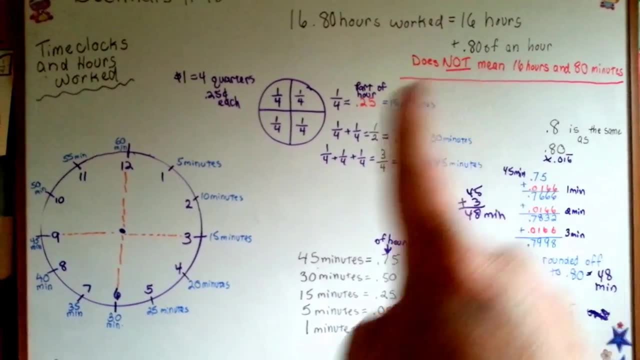 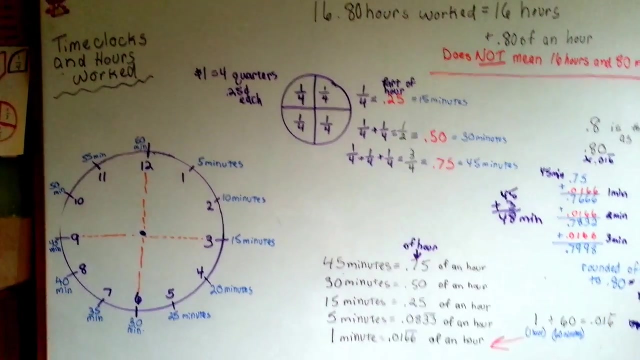 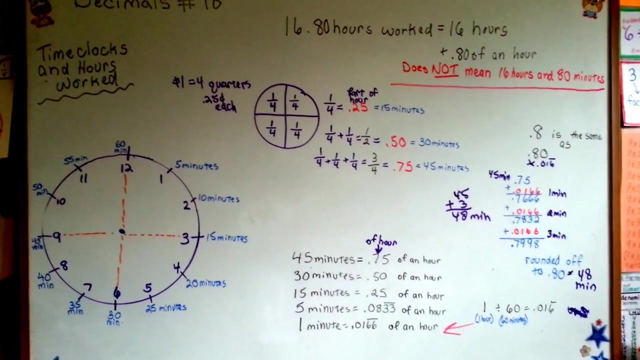 something hours worked. that doesn't mean that it's minutes. That means it's part of an hour and .75 is three-quarters of an hour. right, That is how you figure out your paycheck, your time card and how much you've worked. I hope you understand this. 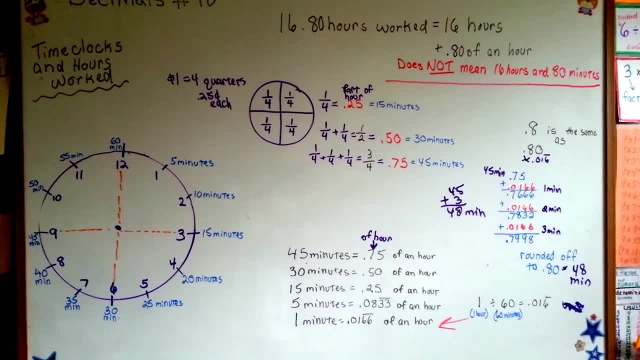 I hope I was clear enough and I hope this helped. See you next video. 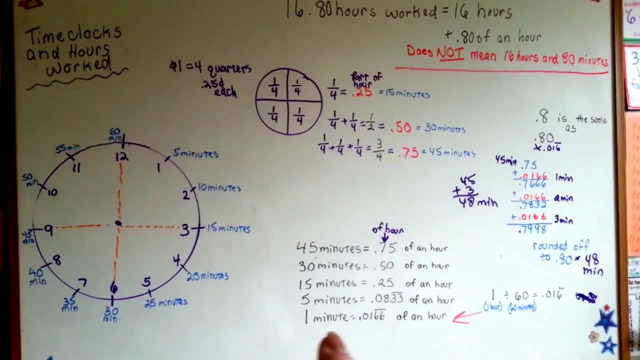 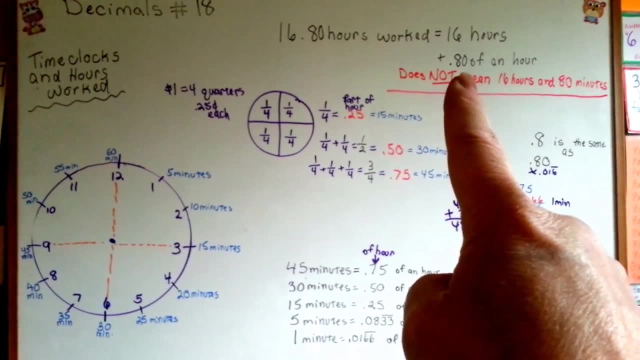 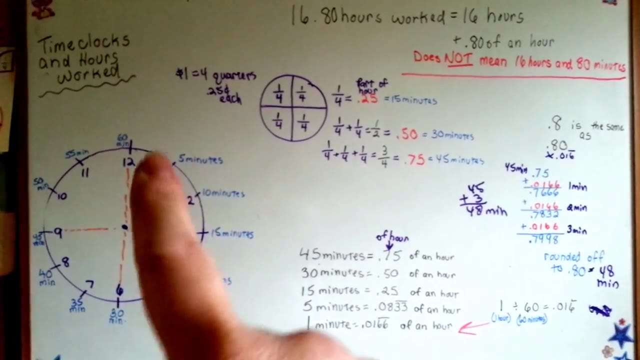 keep in mind that 0.0166 is 1 minute of an hour And when you see 0.something hours worked, that doesn't mean that it's minutes. That means it's part of an hour and 0.75 is 3 quarters of an hour. 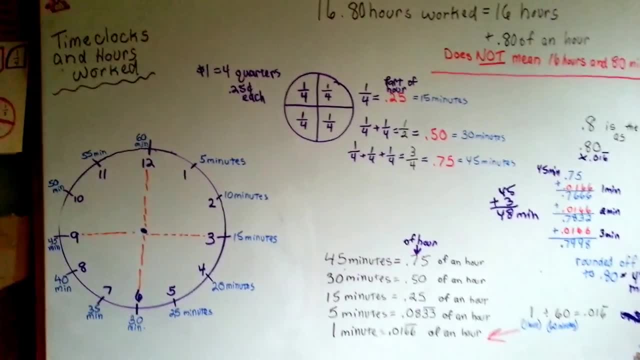 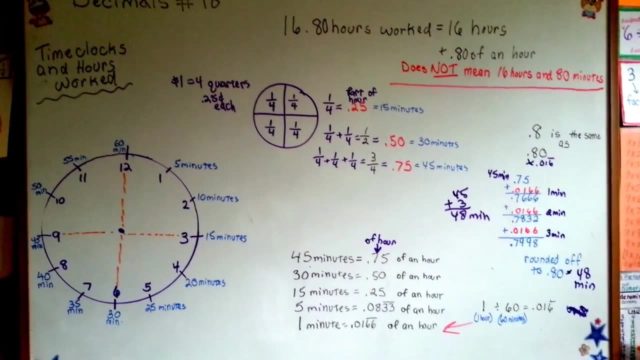 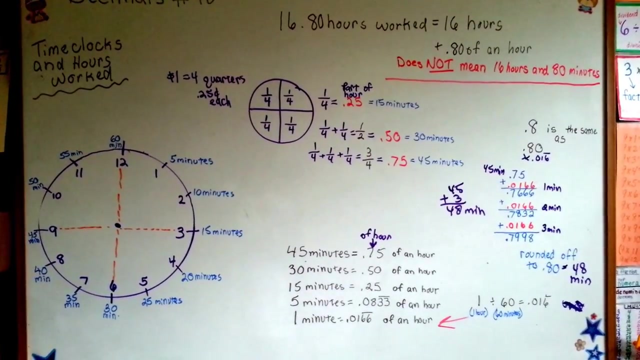 Right, That is how you figure out your paycheck, your time card and how much you've worked. I hope you understand this. I hope I was clear enough and I hope this helped. See you next video. 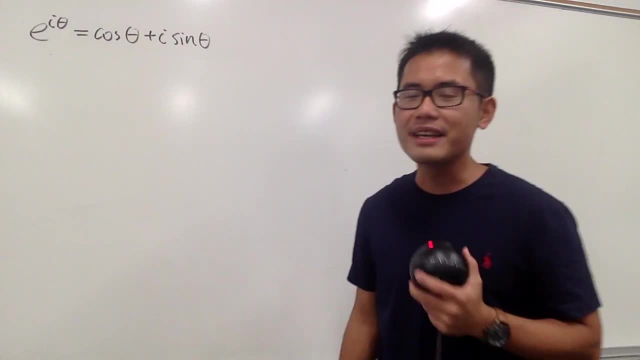 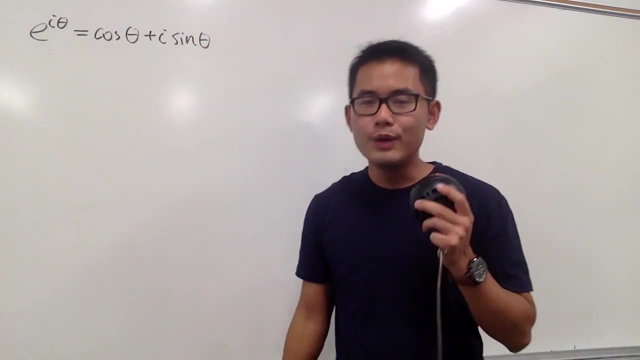 Okay, I'm going to show you guys a complex definition of sine and cosine. and first we're going to start off with the Euler's formula e to the i, theta is equal to cosine theta plus i sine theta, and we are going to plug in z and negative z into theta and we'll come up with two equations. 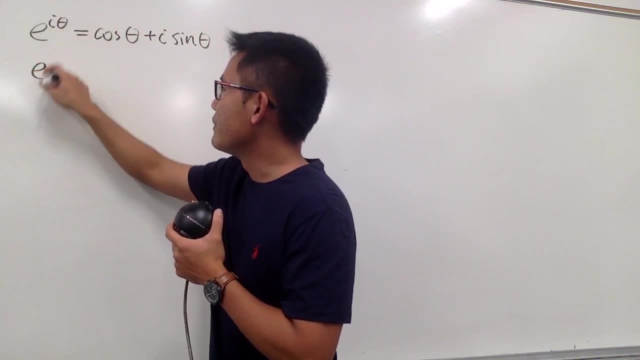 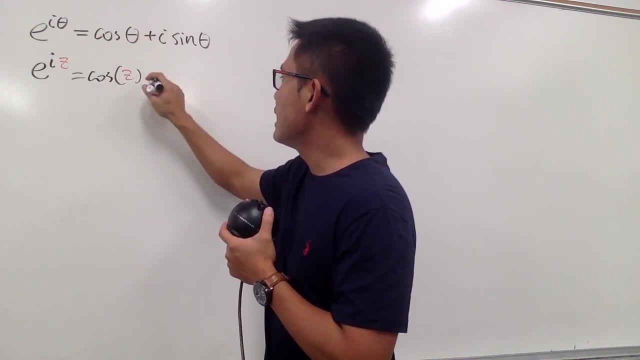 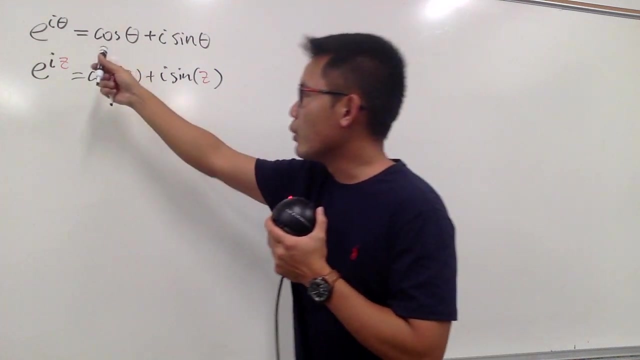 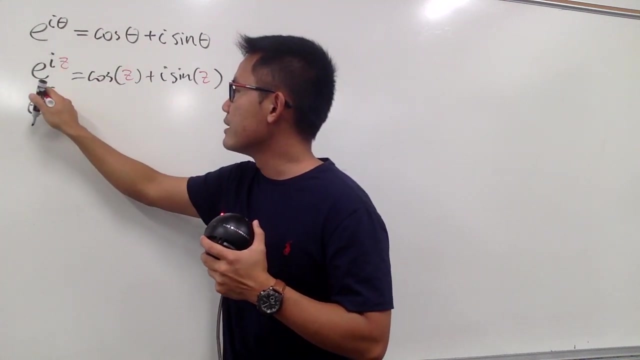 First let me plug in z into all the theta, so we will have e to the i z and this is equal to cosine z, right here, and then plus i sine z like this: and next I will plug in negative z into all the theta, so we will have, right here, e to the i. I plug in negative z right here and let me write it down: negative z like this: 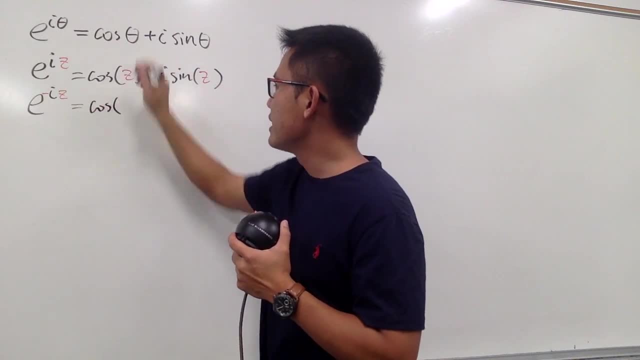 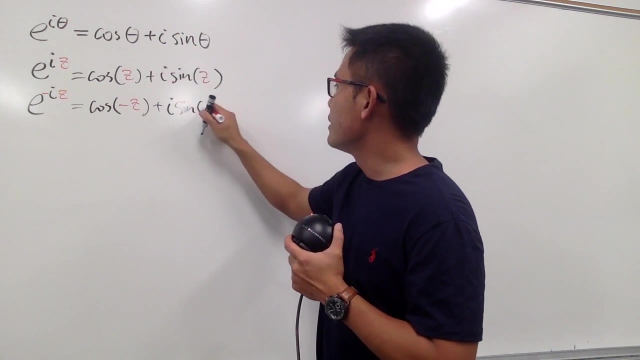 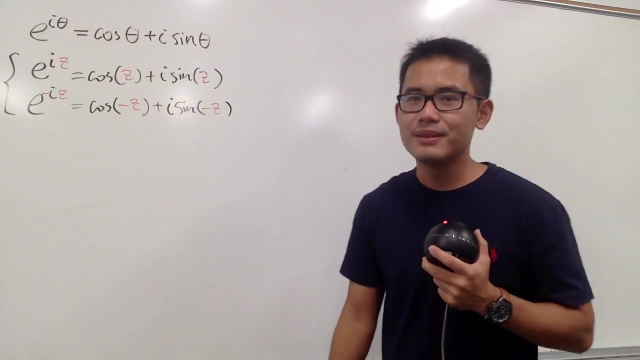 and then we will have equal to cosine negative z, negative z right here into this theta, plus i, and then sine and negative z right here into this theta, all right. And from here we will be able to solve for cosine z and sine z, all right. 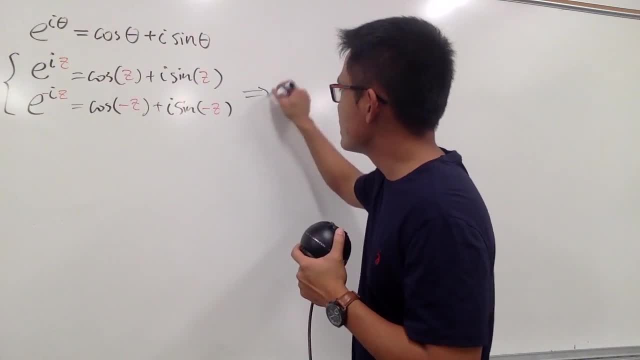 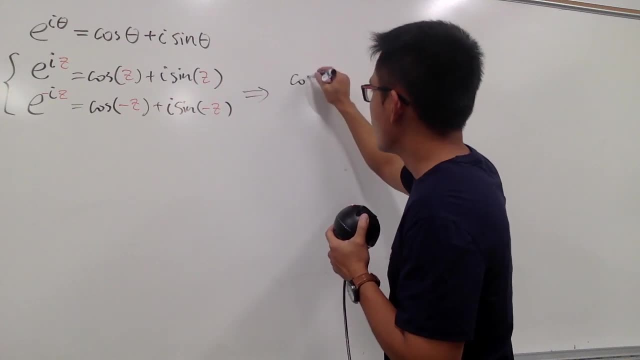 Let's do the cosine z first, and I'm going to just keep the first equation as how it is. I will write down this part first. all right, So we will have cosine z plus i sine z And this: This is equal to e, to the i z right.